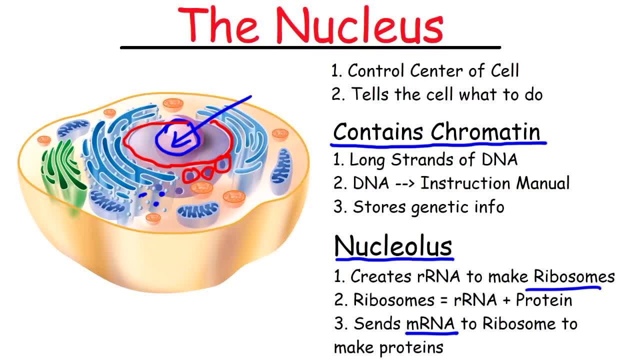 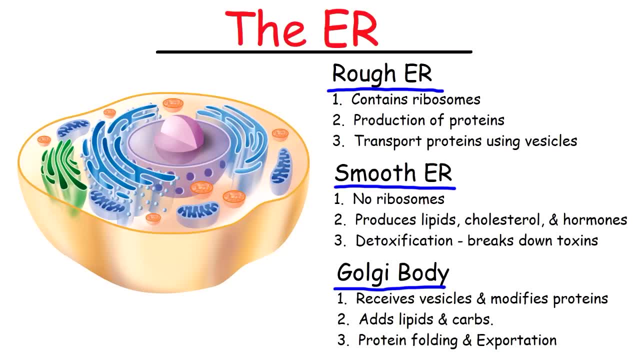 And they allow stuff to go into and out of the cell. So the messenger RNA comes out of the nucleus through those nuclear pores. Now let's talk about the ER, The endoplasmic reticulum. There are two types. The first one is the rough ER, which is all of this in that region. 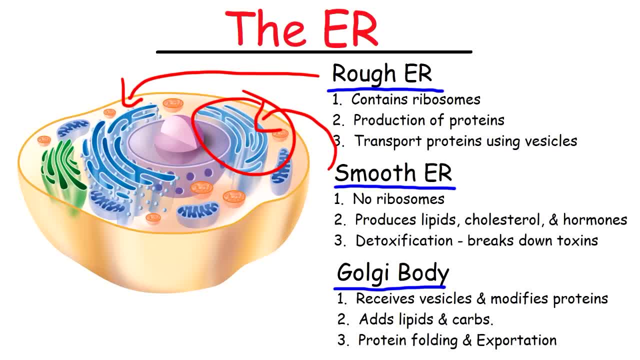 And the second is the smooth ER, which is right here. Now, what do you notice about these two, These two types? What is the difference between them? The rough ER contains ribosomes. The smooth ER does not contain any ribosomes. So the rough ER? it assists in the production of proteins because 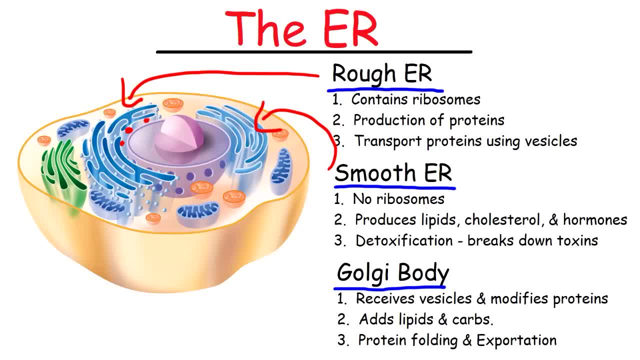 ribosomes. that's what they do: they make proteins. Because the smooth ER doesn't have any ribosomes, it does not make any proteins. However, it does produce lipids, cholesterol and hormones. It also assists in detoxification, which means it breaks down toxins And the way 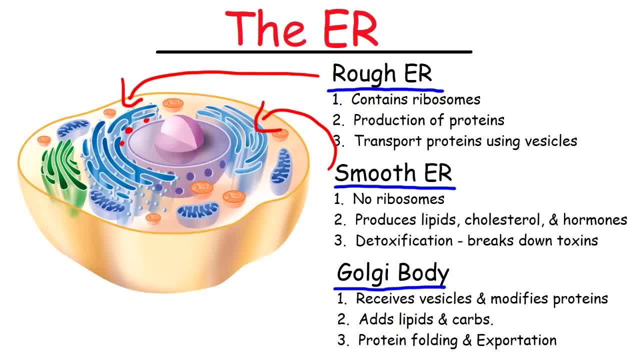 it does so is by making these molecules more water-soluble, so that they can be easily removed from the body or excreted through the urine. Now let's go back to the rough ER. So once, the rough ER by means of the ribosomes. once they make the proteins, the proteins are enclosed in. 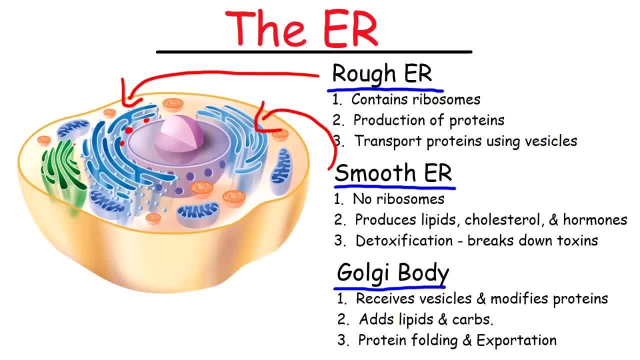 a vesicle And those vesicles get transported to the Golgi body, which is right there Now, the Golgi body. it receives the vesicles and it modifies the proteins that are in the vesicles, And the way it does so is by adding lipids and carbs to the proteins, And it can also fold the protein. It 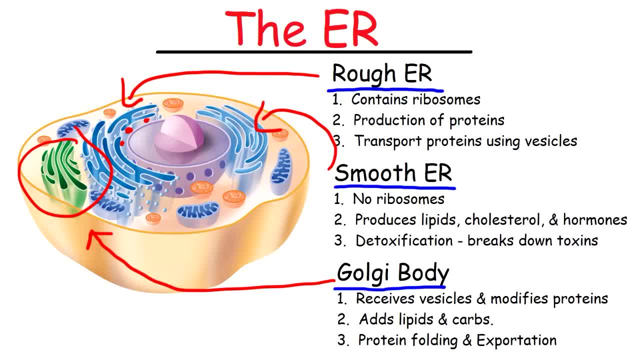 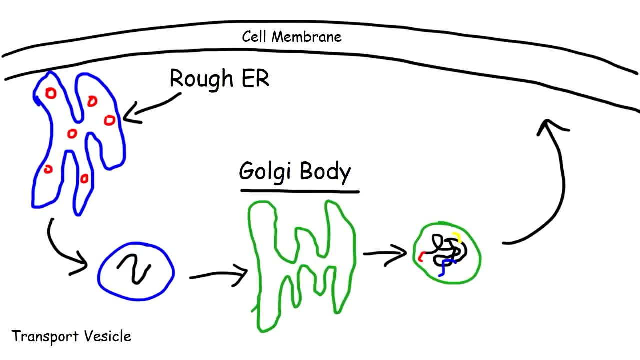 can give it the proper shape, because the function of a protein is dependent on its shape. So once it modifies and processes the proteins, it exports the proteins out of the cell. So here is a visual illustration of what happens to a protein in the cell. Now. granted, my drawing is not the best. This is an educational 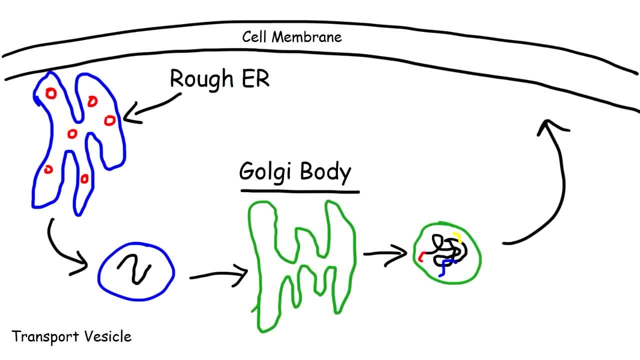 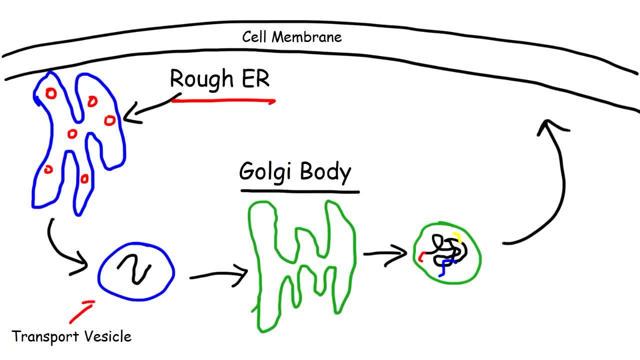 The protein. it leaves the rough ER by means of a transport vesicle And you can see the protein inside of this vesicle And it goes to the Golgi body for processing and modification. So, looking at the protein now, you can see that it has a different shape. At the same time, you can see 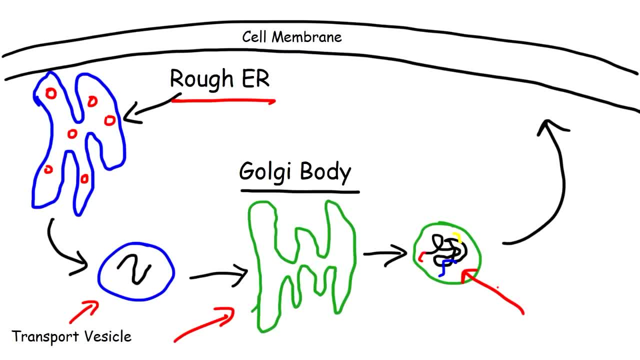 different colors added to it. So this represents the lipids and the carbs added to the protein. So once the protein has been tagged with those extra molecules, it gets exported out of the cell So it travels to the cell membrane where it leaves the cell. 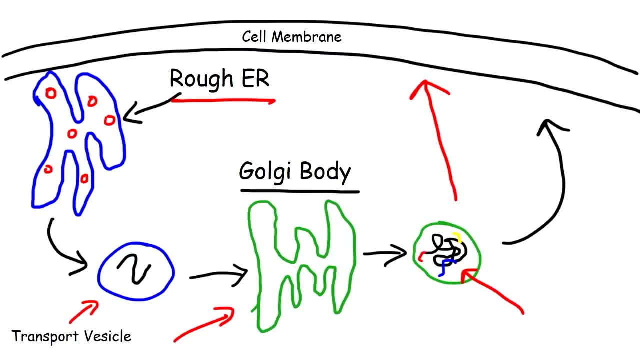 to perform the function that it needs to do Now: the transport vesicle that surrounds the protein. it fuses with the cell membrane And so it becomes part of the cell membrane, causing the membrane to expand or basically causing the cell to grow. 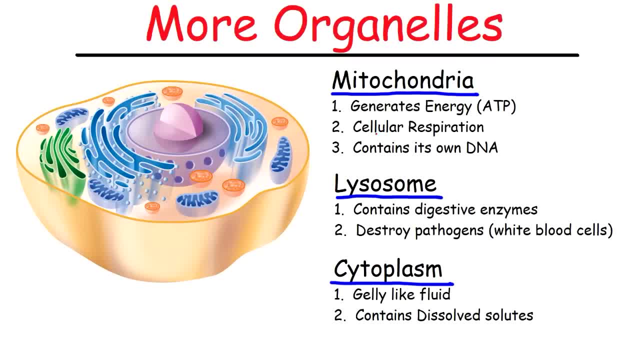 Now let's talk about some other organelles that you need to know. The next one is the mitochondria. Now, the mitochondria has its own separate DNA. It's different from the DNA of the cell And its job is to perform cellular respiration. In that process, it takes the energy stored in fats and 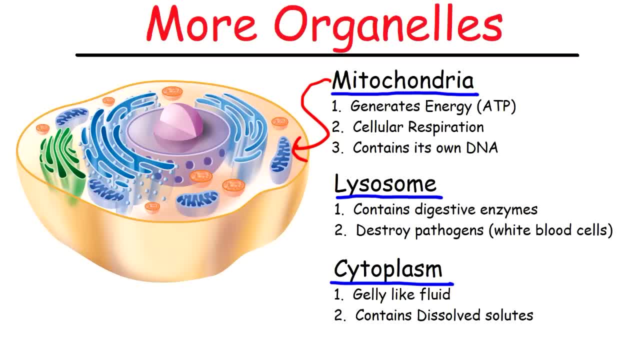 carbohydrates and converts it to a molecule known as ATP, adenosine triphosphate. Next up we have the lysosome. Now, the lysosome which is here. its purpose is to break down the cell's food. It contains digestive enzymes And in white blood cells it can also destroy pathogens When 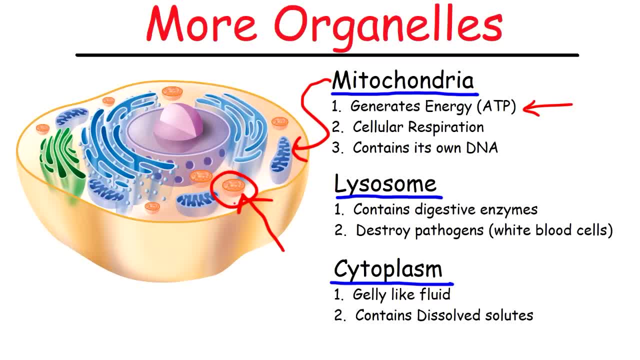 a white blood cell engulf a pathogen. in a process known as phagocytosis- the lysosomes in those white blood cells- it can break down those pathogens or disease-causing agents into smaller stuff that could be used or recycled by the cell. Next up we have the cytoplasm. The cytoplasm is basically. 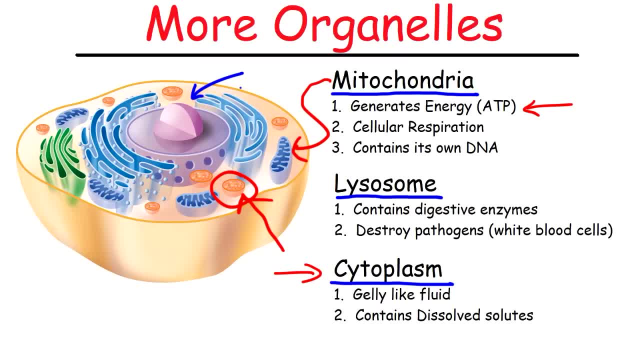 the jelly-like fluid that is in the cell, So all of the organelles. they're dissolved in the cytoplasm. The cytoplasm contains solutes like salts, electrolytes and other stuff like carbohydrates, lipids and free-floating ribosomes and things like that. Now let's talk about the. 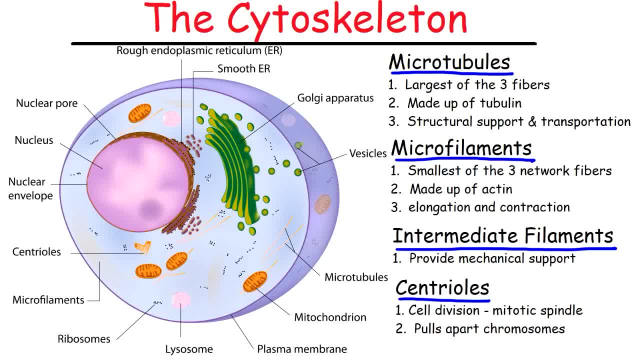 cytoskeleton. The function of the cytoskeleton is to maintain the shape of the cell. At the same time, it also provides structural support. Now, the cytoskeleton consists of a network of three fibers, The first of which is the microtubules, The second is the microfilaments And the third one the intermediate filaments. Now, 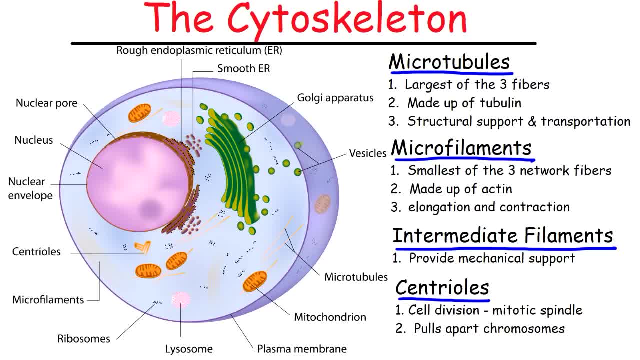 how can we identify them in the cell? The microtubules is the largest of the three fibers. The microfilaments is the smallest of the three fibers. The intermediate filaments are somewhere in between the microtubules and the microfilaments. Now, this picture really doesn't. 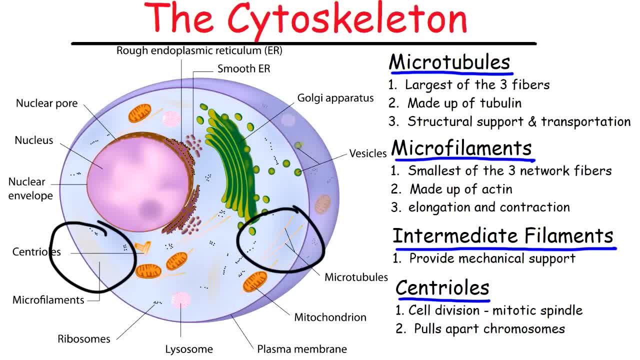 show it, But just know that the intermediate filaments are in between and they provide mechanical support to the cell. Now, the microtubules: they're made up of a protein called tubulin, And the microfilaments: they're made up of a protein called actin. The microtubules: 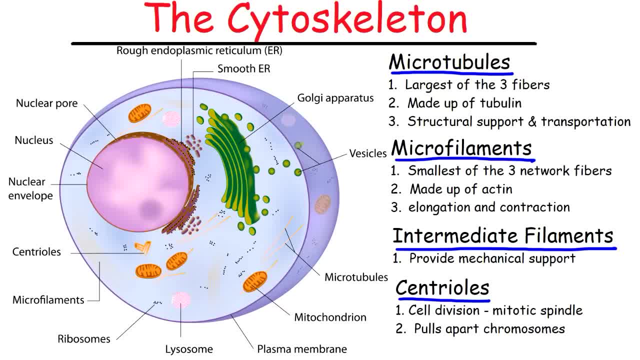 their purpose is to provide structural support and transportation services to the cell, So vesicles. they can move from one part of the cell to another part by means of the microtubules, The microfilaments. they're involved in elongation and contraction, So they assist the cell to move. Next up we have the centrioles. 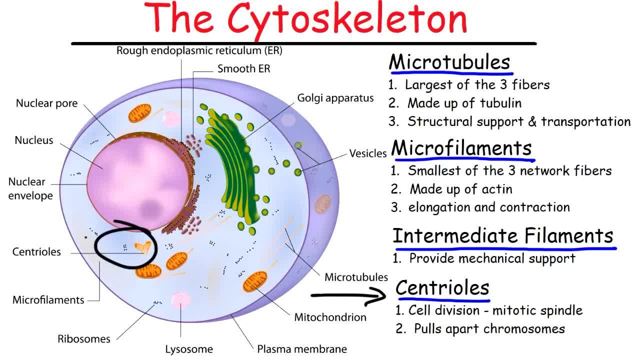 And here it is in the diagram. The centrioles are active during cell division, And during that time they form something known as the mitotic spindle, which consists of microtubules, And what it does is, during cell division, it pulls apart the chromosomes, thus allowing the cell to be split. 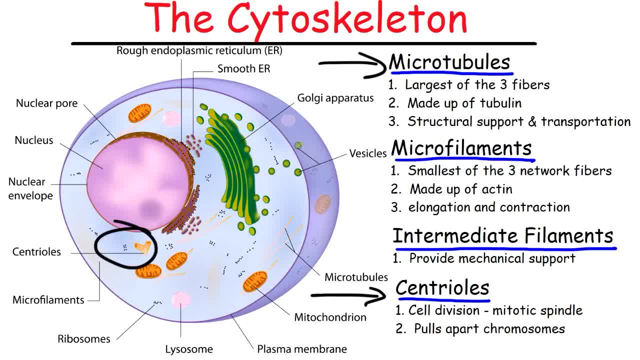 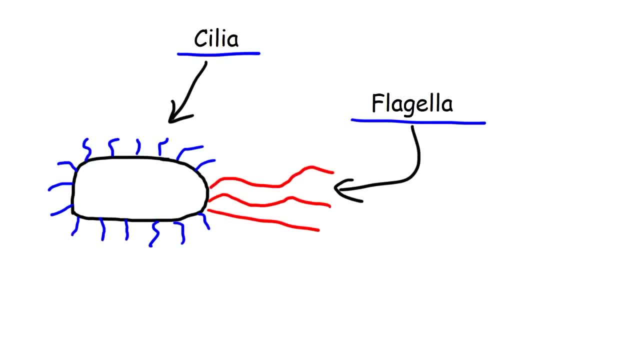 into two. The chromosomes are basically a condensed version of chromatin, So they form during cell division. Now here are some other terms that you need to be familiar with: Cilia and flagella. These also play a role in the movement of a cell. Now, cilia consists of tiny, short hair-like structures. 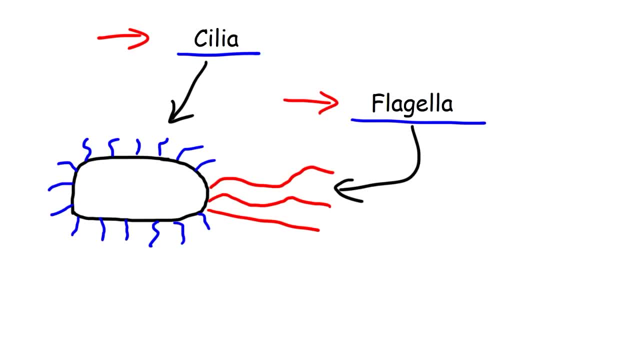 And notice that there's many of them. Flagella consists of long, whip-like structures, And there's only a few of them, And so the flagella can propel a cell forward from one location to another. Now, these two structures: they're made up of microtubules. 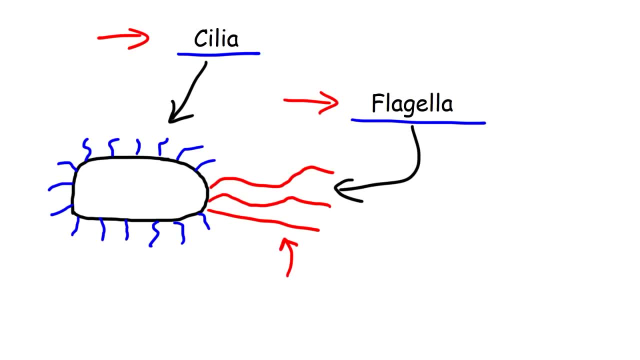 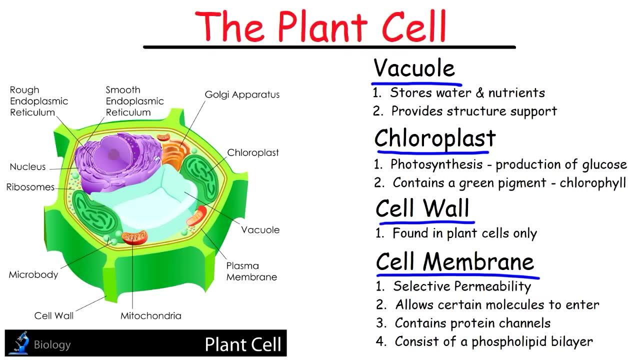 So microtubules. they're very useful in the movement of a cell. So far we've been talking about animal cells, But now let's talk about the plant cell, Because, even though they are similar, the plant cell has some characteristics that are not found. 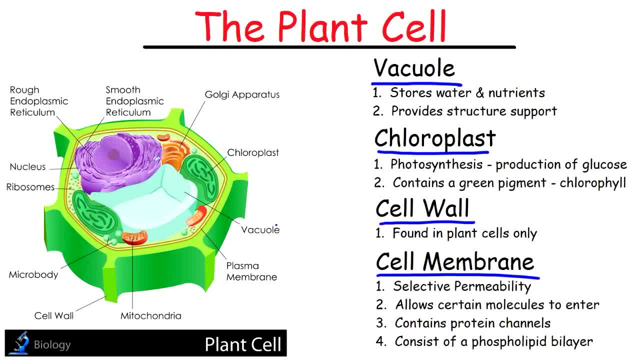 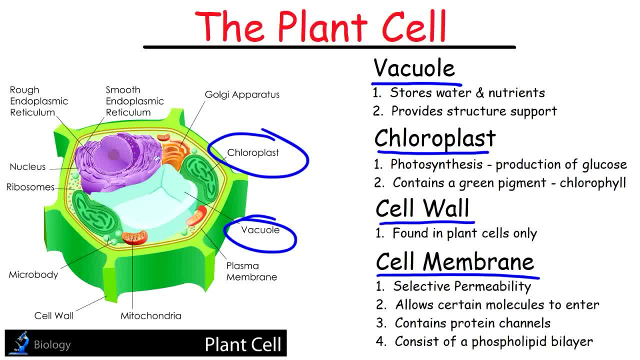 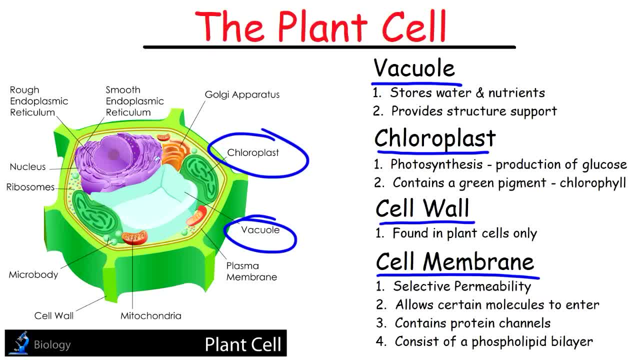 Now the chloroplast is green due to a pigment known as chlorophyll, which plays a role in photosynthesis. Photosynthesis is a process by which the plant takes sunlight, carbon dioxide and water, and it produces glucose and oxygen gas. 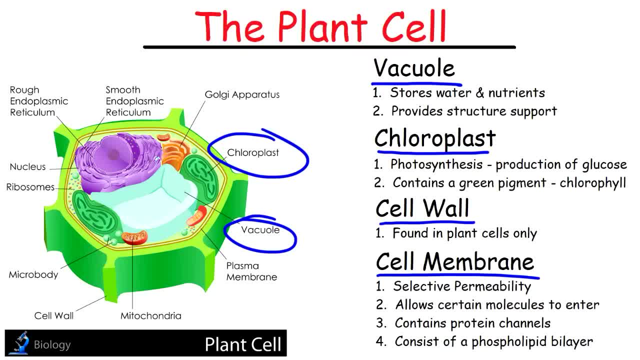 Another feature that's present in plant cells but not in animal cells, is the presence of a cell wall. Now, both the animal cell and the plant cell, they both contain a cell membrane. The cell membrane consists of a phospholipid bilayer And it has a property known as selective permeability.